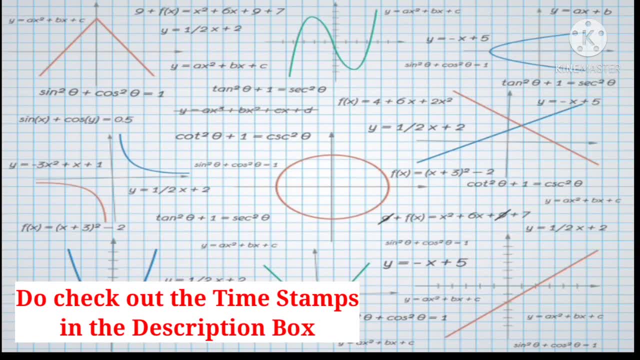 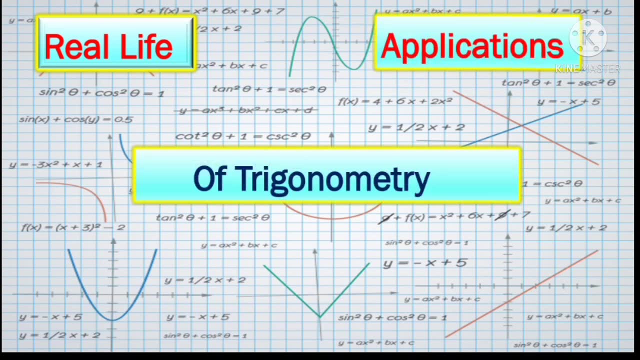 Hello everyone, In today's video we will be exploring the real life applications of trigonometry. and, friends, you will realize that trigonometry is not just another chapter in maths, but is also an invaluable tool that is widely used. So let's start A very common application. 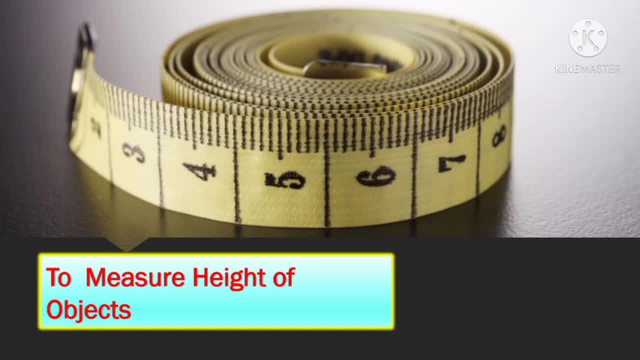 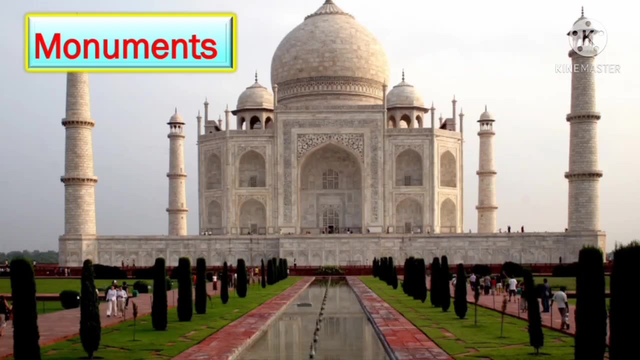 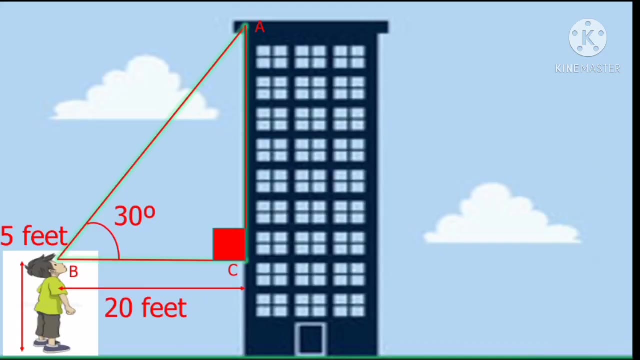 of trigonometry is to measure heights of objects. So, friends, you would have often wondered that how do we know the heights of tall mountains and ancient monuments and even skyscrapers? Well, it's all made possible due to trigonometric concepts, and I'll show you how. Suppose you want to find. 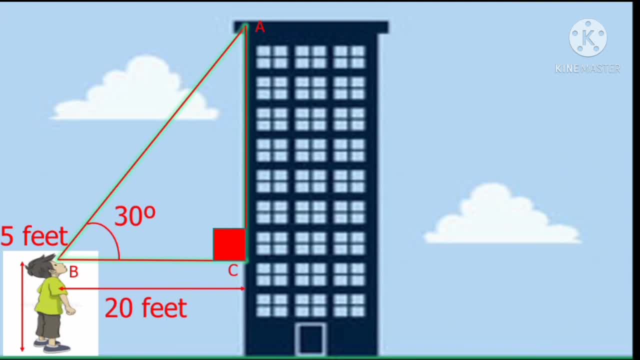 the height of a nearby building and you are at a distance of 20 feet away from it. Let's suppose your height to be 5 feet. friends, Now just look at the top of the building and note down the angle that your line of sight makes with the horizontal. Let's suppose it is 30 degrees. So did you see? 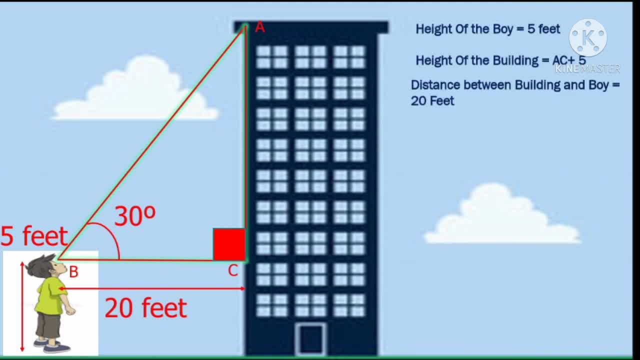 that you are getting a beautiful right angle triangle friends, and wherever you have right angle triangles you can use all your trigonometry concepts. So we can say that tang 30 is the opposite side upon the adjacent side, that is, AC upon BC. So just substituting all the values that 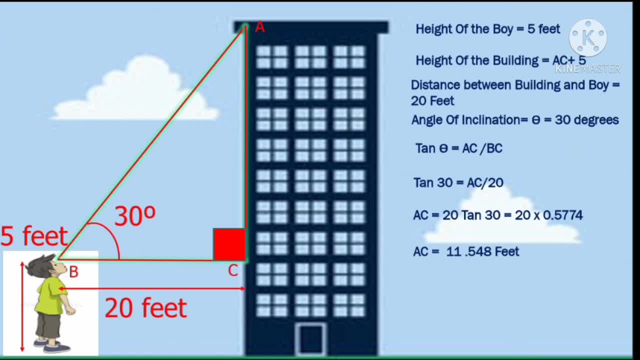 we have, we'll find out that AC is 11.548 feet, but the height of the building is going to be AC plus your height, So it will be 16.548 feet. So, friends, I hope you have found this video helpful. I hope you understood the concept that is used to measure heights of buildings and other 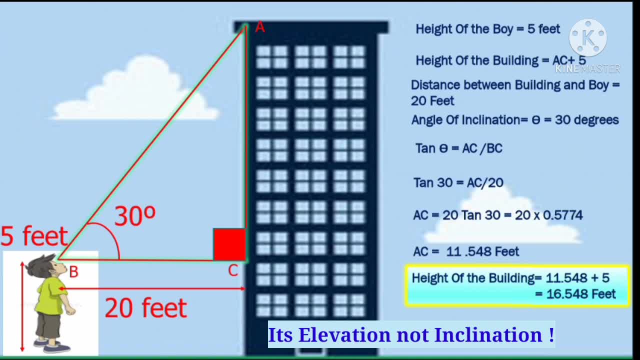 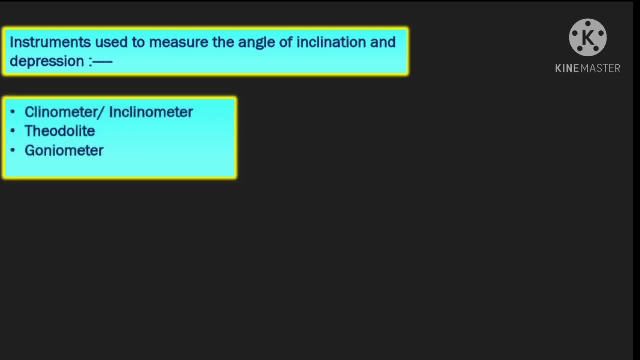 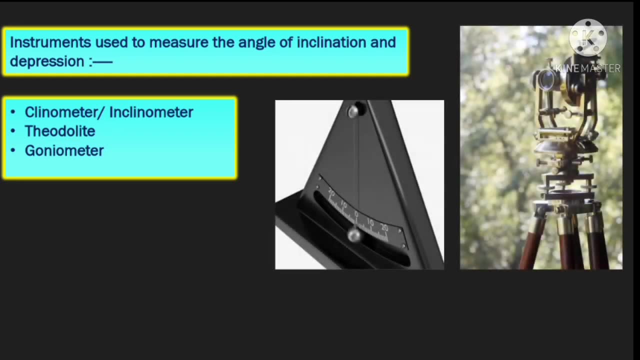 structures. Now, in case you're wondering: how do I find the angle of inclination? Well, friends, there are numerous instruments that are available and that are widely used, namely the clinometer or the inclinometer, theodolite, goniometer, and you can even make DIY clinometers, So do go ahead. 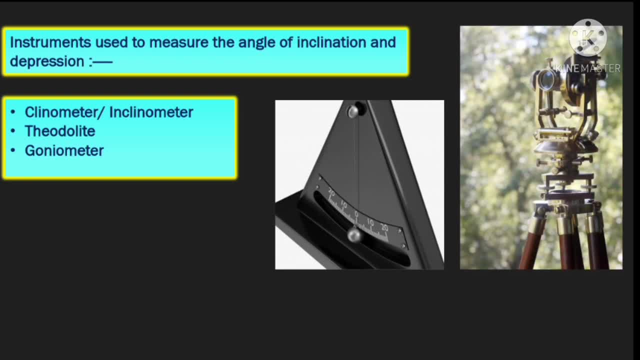 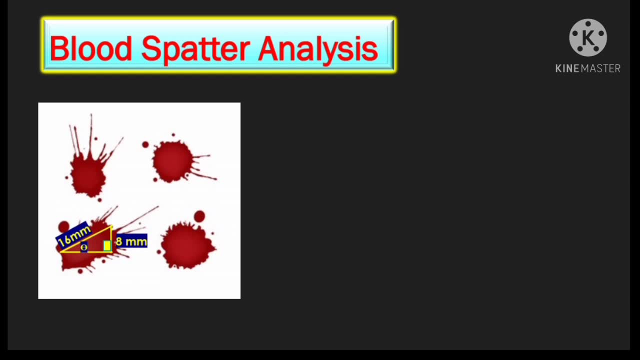 try them out and find heights of some nearby buildings. Another important application of trigonometry is in criminology. So, friends, trigonometry is very useful in blood spatter analysis. Now, that is nothing but the interpretation of blood stain patterns. Now, this is done mainly. 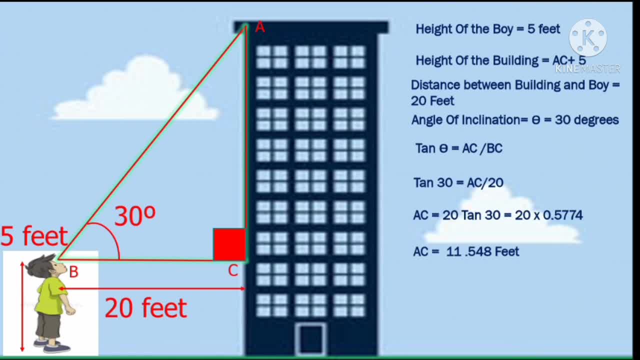 we have, we'll find out that AC is 11.548 feet, but the height of the building is going to be AC plus your height, So it will be 16.548 feet. So, friends, I hope you have found this video helpful. I hope you understood the concept that is used to measure heights of buildings and other 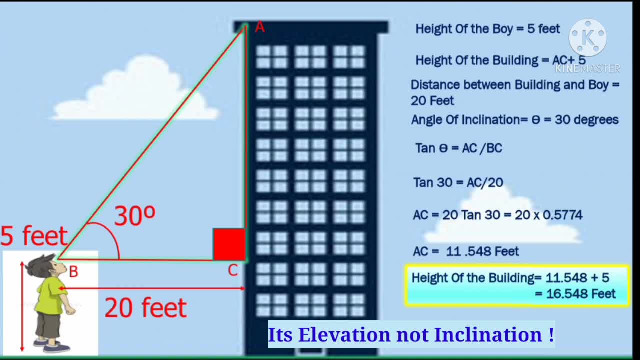 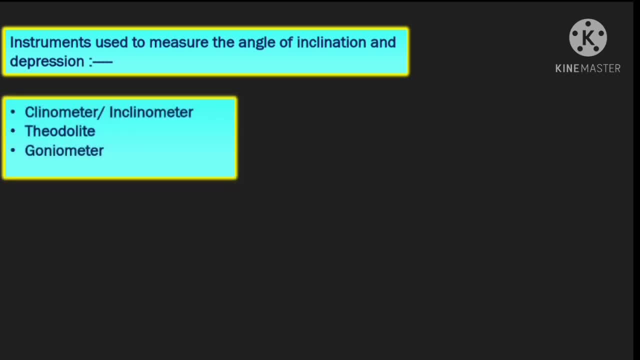 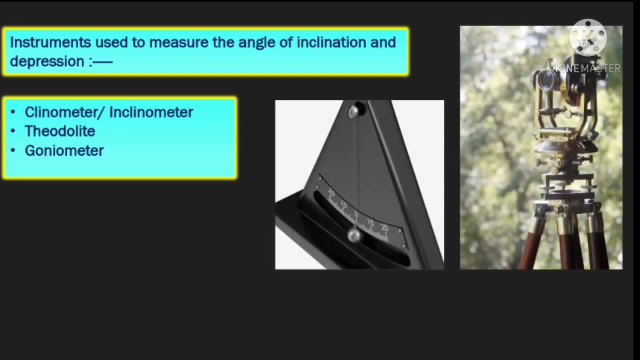 structures. Now, in case you're wondering: how do I find the angle of inclination? Well, friends, there are numerous instruments that are available and that are widely used, namely the clinometer or the inclinometer, theodolite, goniometer, and you can even make DIY clinometers, So do go ahead. 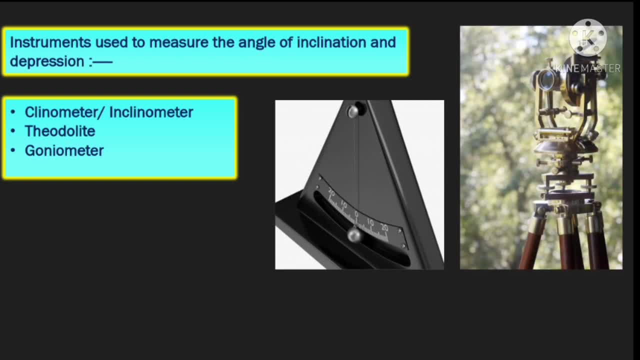 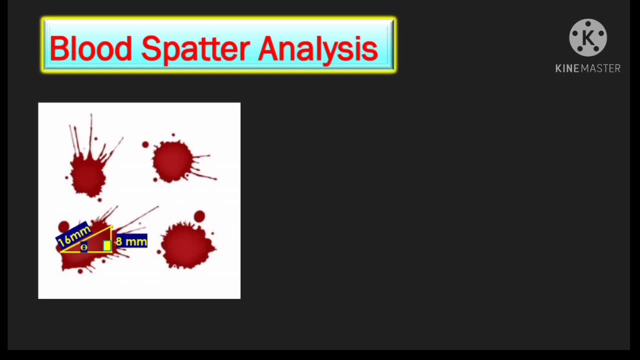 try them out and find heights of some nearby buildings. Another important application of trigonometry is in criminology. So, friends, trigonometry is very useful in blood spatter analysis. Now, that is nothing but the interpretation of blood stain patterns. Now, this is done mainly. 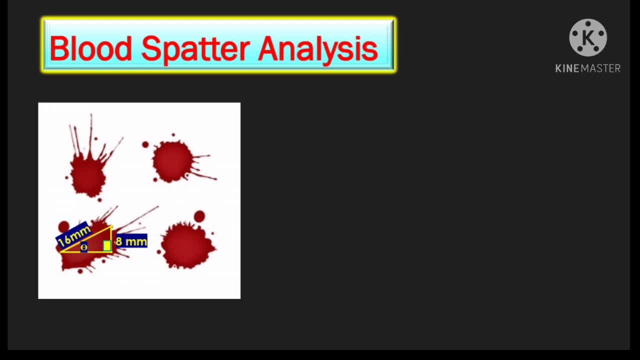 by forensic experts to reconstruct the scene of crime or accident and also to determine where the blood originated from. So let's suppose the width of a blood stain is 8 millimeters and its length is 16 millimeters. Then they find the angle of impact. Now, that angle of impact? 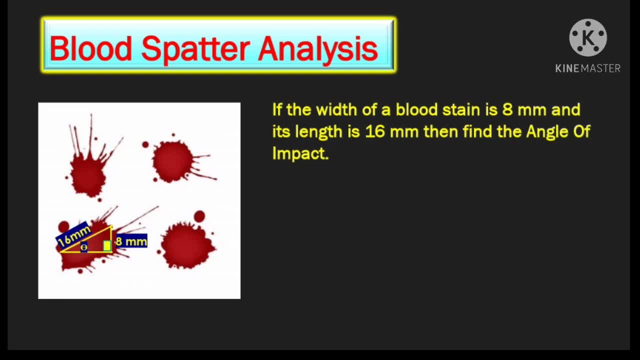 tells us the angle at which the blood hit the surface. So in this case, did you see, you're getting a right angle triangle, So you can use the trigonometric concepts, So we can say that sine theta is opposite side upon the hypotenuse, So sine theta is 8 upon 16, so your angle of impact is 30 degrees. 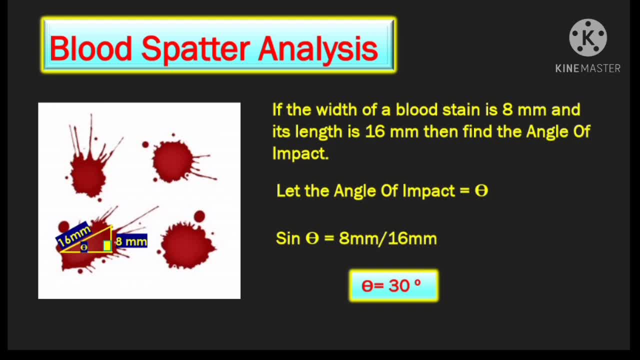 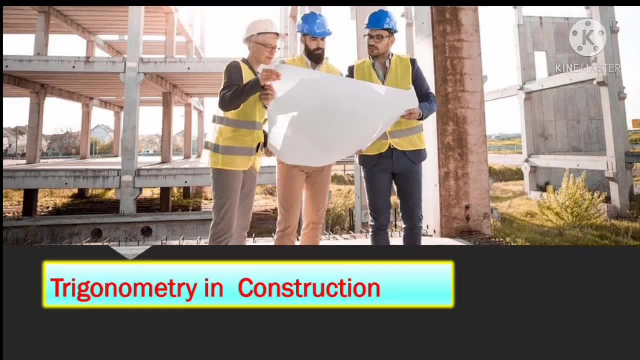 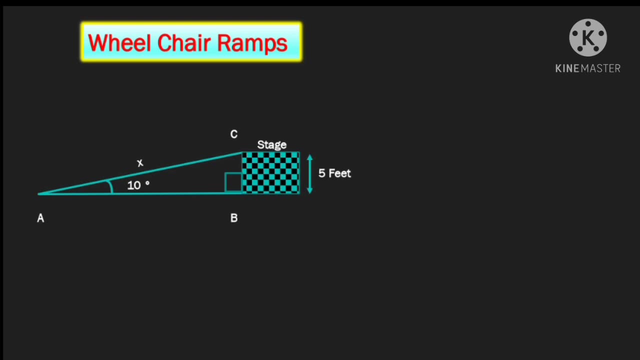 So with this angle the forensic experts can do further analysis. So in this way trigonometry is very useful in criminology. The next application of trigonometry is in construction. Friends, let's take an example where you have to construct a wheelchair ramp for a stage of height 5 feet. 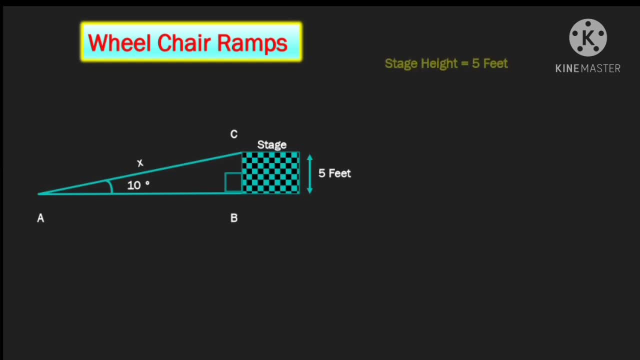 And suppose the ramp has to be at an angle of 10 degrees for maximum safety. Now you need to find the length of the ramp, So let that be equal to x. So, friends, did you see that you're again getting a right angle triangle, which means you can use the trigonometric concepts. So sine 10 degrees. 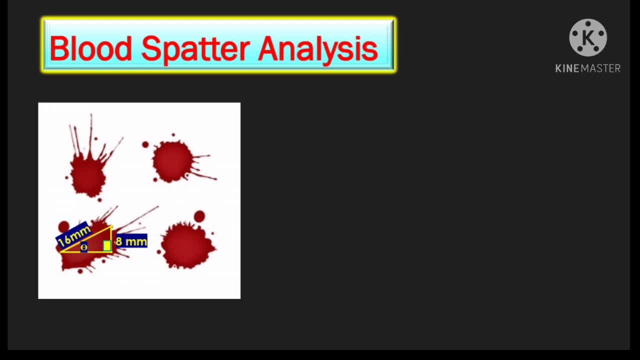 by forensic experts to reconstruct the scene of crime or accident and also to determine where the blood originated from. So let's suppose the width of a blood stain is 8 millimeters and its length is 16 millimeters. Then they find the angle of impact. Now, that angle of impact? 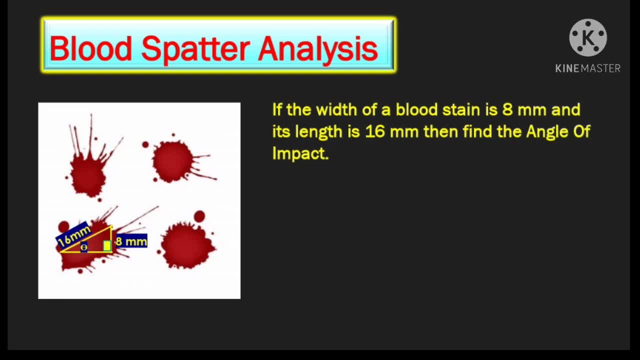 tells us the angle at which the blood hit the surface. So in this case, did you see, you're getting a right angle triangle, So you can use the trigonometric concepts, So we can say that sine theta is opposite side upon the hypotenuse, So sine theta is 8 upon 16.. So your angle of impact is 30 degrees. 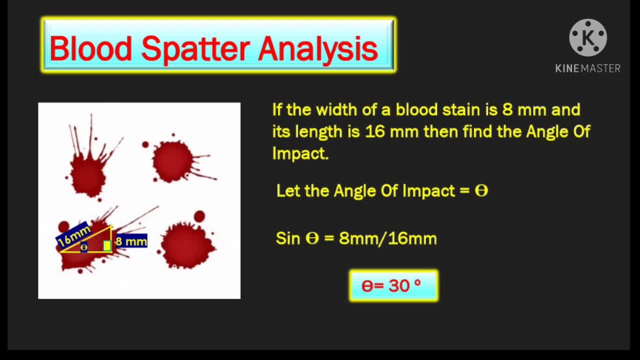 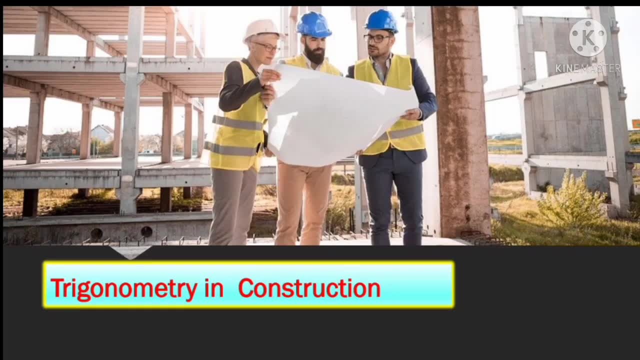 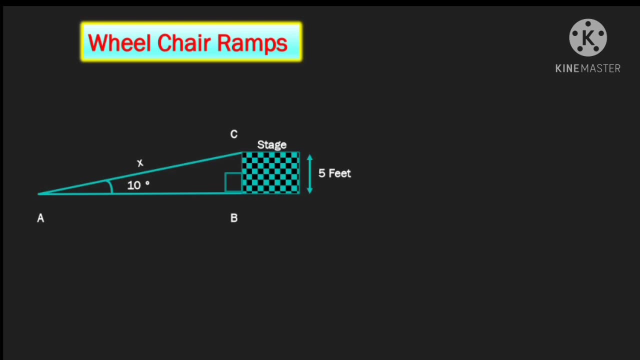 So with this angle the forensic experts can do further analysis. So in this way trigonometry is very useful in criminology. The next application of trigonometry is in construction. Friends, let's take an example where you have to construct a wheelchair ramp for a stage of height 5 feet, And suppose the 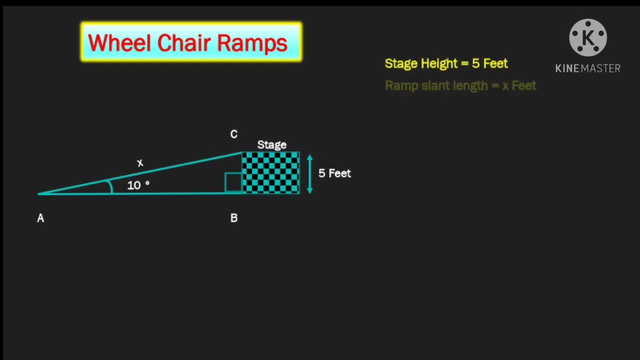 ramp has to be at an angle of 10 degrees for maximum safety. Now you need to find the length of the ramp, So let that be equal to x. So, friends, did you see that you're again getting a right angle triangle, which means you can use the trigonometric concepts. So sine 10 degrees. 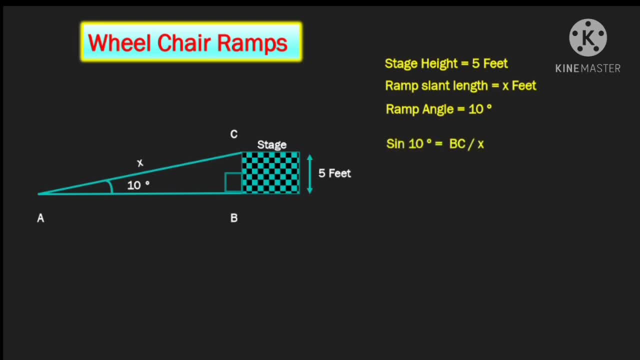 Is nothing but the opposite side upon the hypotenuse, That is, bc upon x. So just need to substitute the values and you will see that x is 28.8 feet. That is, the wheelchair ramp length is 28.8 feet. And, friends, this is just one of the numerous ways in which trigonometry is so useful. 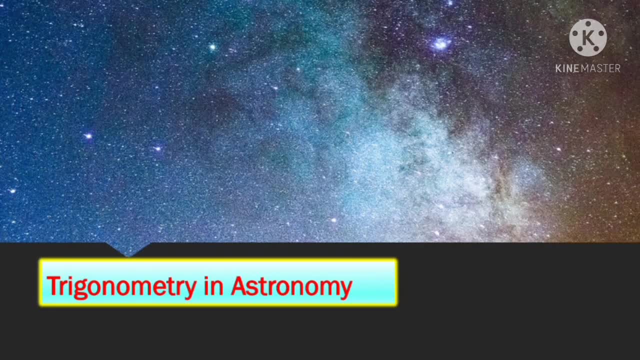 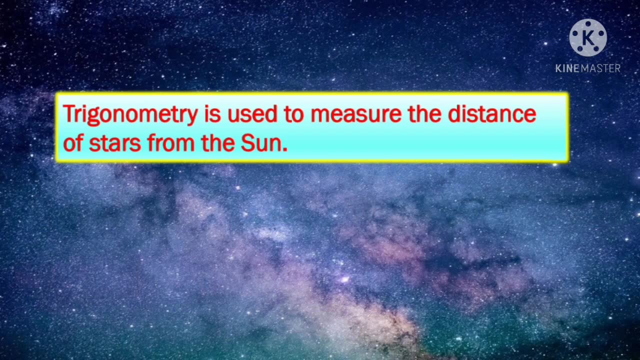 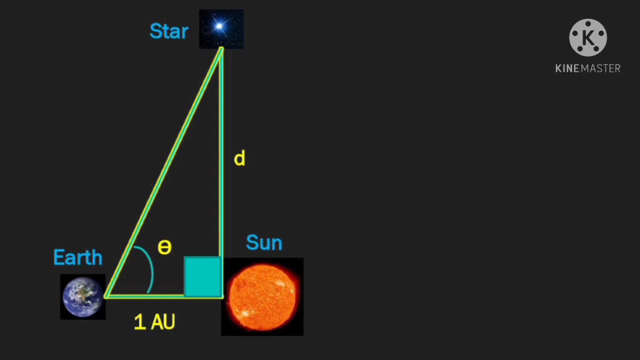 in construction. Trigonometry and astronomy are inseparable, and trigonometry is very widely used, especially to measure the distance of stars from the sun. Suppose, friends, you want to find the distance between sun and a particular star, Let's call that distance as d. Now we already know the. 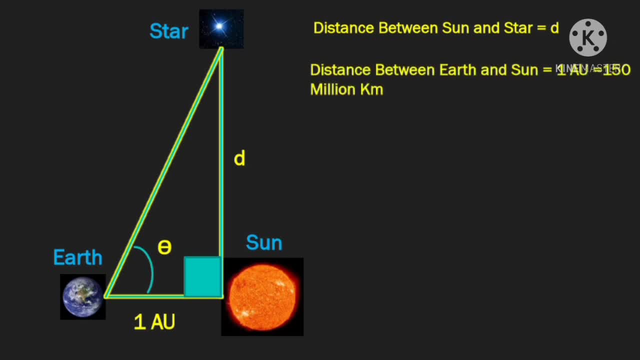 distance between sun and earth to be one astronomical unit, which is nothing but approximately 150 million kilometers. Now, when the distance between the sun and the star, and the sun and earth when they are perpendicular to each other, at that time you need to observe the star. 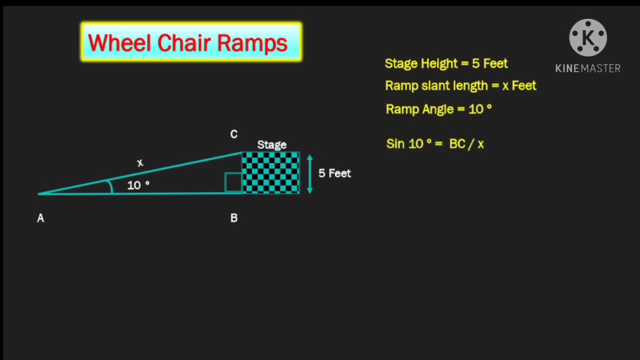 Is nothing but the opposite side upon the hypotenuse, That is, bc upon x. So just need to substitute the values and you will see that x is 28.8 feet. That is, the wheelchair ramp length is 28.8 feet. And, friends, this is just one of the numerous ways in which trigonometry is so useful in construction. 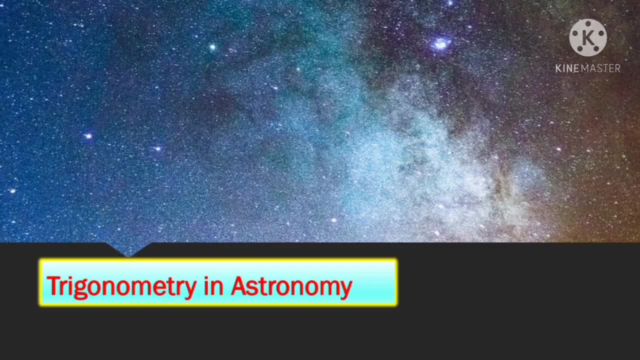 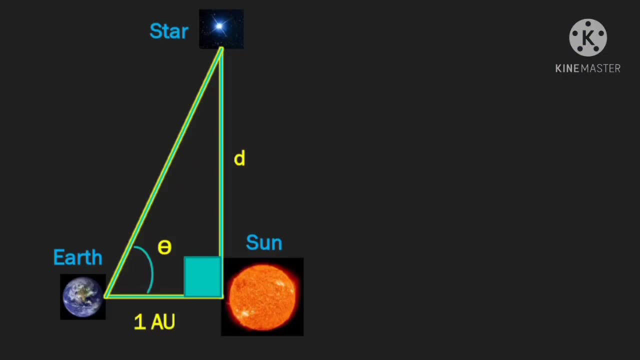 Trigonometry and astronomy are inseparable, and trigonometry is very widely used over there, Especially to measure the distance of stars from the sun. Suppose, friends, you want to find the distance between sun and a particular star, Let's call that distance as d. Now we already know the distance between sun and earth to be. 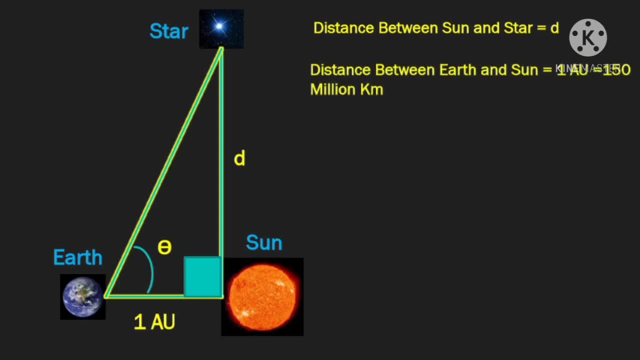 one astronomical unit which is nothing but approximately 150 million kilometers. Now, when the distance between the sun and the star and the sun and earth, when they are perpendicular to each other, At that time you need to observe the star and note down the angle of inclination. 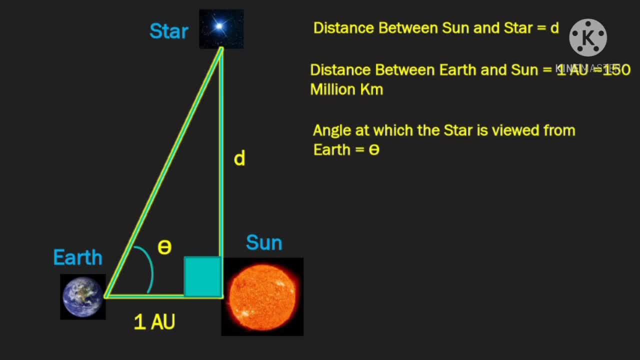 Let that be theta, and let's say that the theta was 60 degrees. So, friends, did you see that again you are getting a right angled triangle over here, so you can use the trigonometric concepts. so we will say that tan theta is opposite upon adjacent, which is d upon one astronomical unit. so for this case, 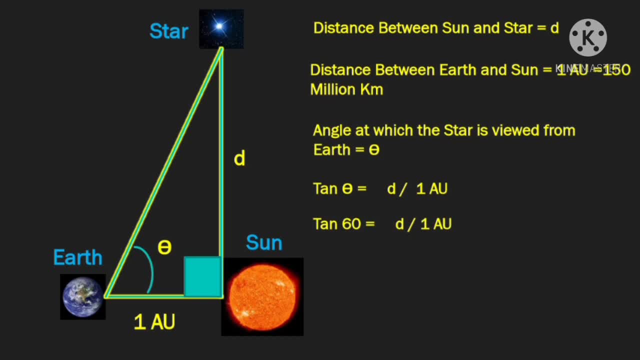 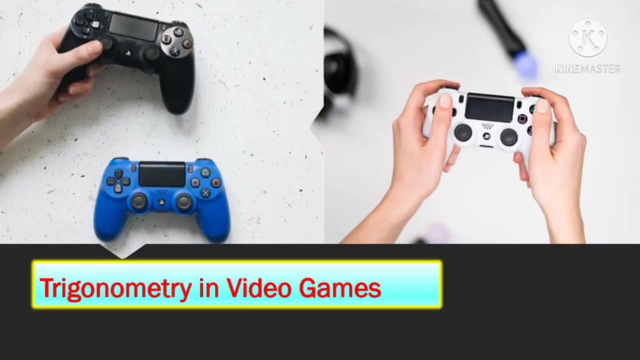 we will take theta as 60. just need to substitute the values and you will see that the distance between the sun and the star is 1.7321 astronomical unit. So, friends, you can just imagine how important trigonometry is in astronomy. moving on to the next application, trigonometry takes: 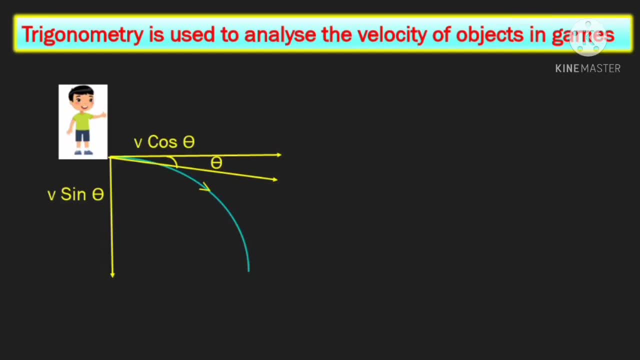 video gaming to the next level. let's see how, suppose friends. then again, if a character is moving at a certain velocity, say v meters per second, then while actually writing the code, we need to split this velocity vector into two components. one is the horizontal component, or v cos theta, and the other is the vertical component, or v sine theta. so by manipulating, 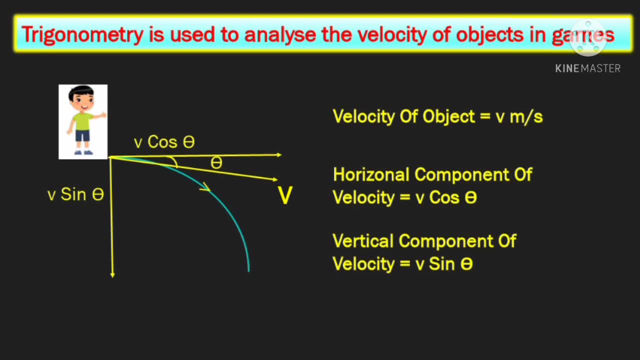 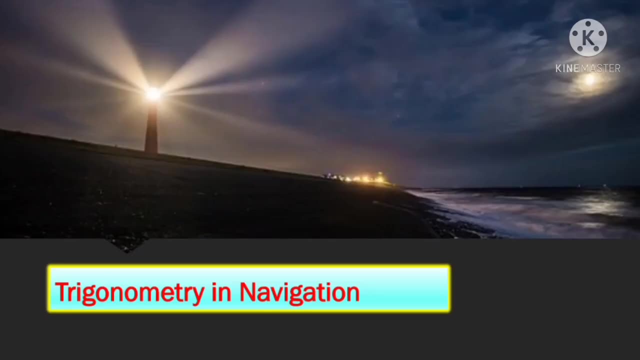 the values of v cos theta and v sine theta we get the net velocity vector of the object. so knowledge of trigonometry is very much needed while writing the codes of these programs. so trigonometry is indeed handy in video gaming. the next application of trigonometry is in navigation. so, friends, let's. 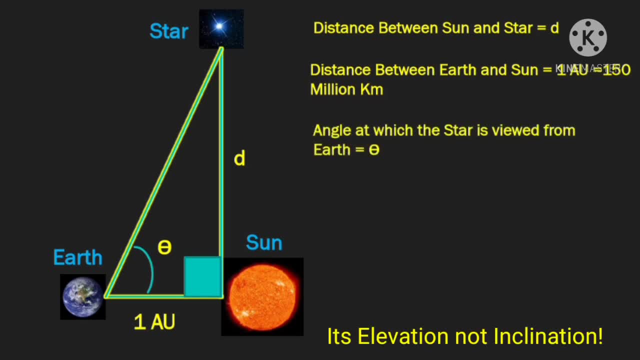 and note down the angle of inclination. Let that be theta, and let's say that that theta was 60 degrees. So, friends, did you see that? again you are getting a right angle triangle over here, So you can use the trigonometric concepts. So we 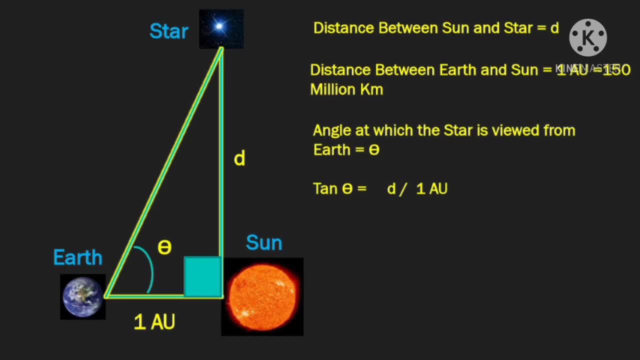 will say that tan theta is opposite upon adjacent, which is d upon one astronomical unit. So for this case we'll take theta as 60. Just need to substitute the values and you'll see that the distance between the sun and the star is 1.7321 astronomical unit. So, friends, you can. 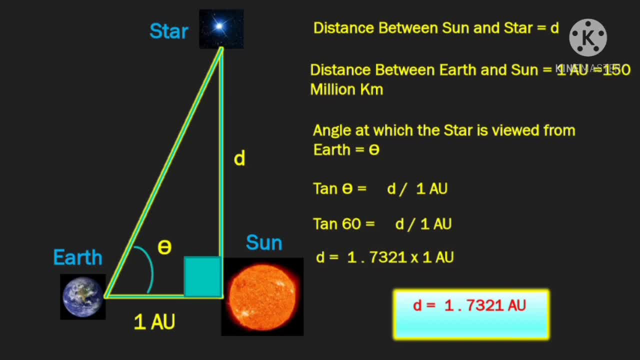 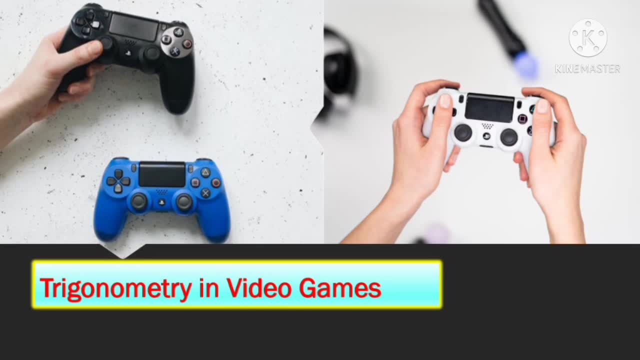 call this as d theta, which you know. that is the basic angle. we can be able to do that. So you take theta as 20.. You can substitute the values and you'll say that you can see that the distance between the sun and the star has come with the breast to the centre. So you can. 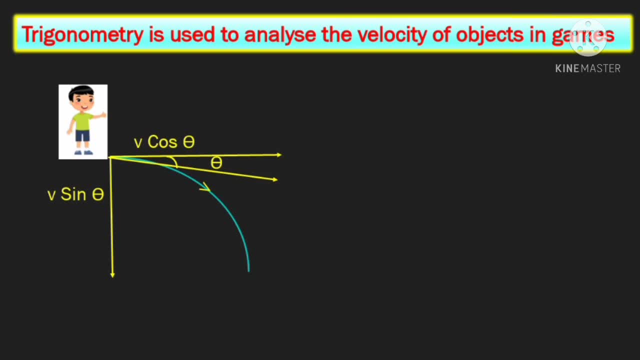 say that the distance between both the stars and the stars is 1.7321 astronomical unit. Now in this application we will be able to do some trigonometry questions. So what are the trigonometric questions we are going to ask the student in this application? So first question: 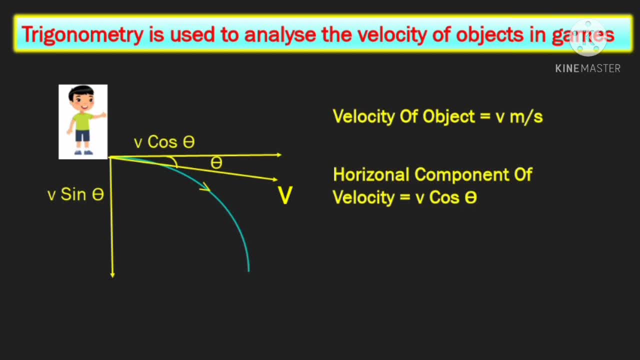 the horizontal component, or V cos theta, and the other is the vertical component, or V sine theta. So by manipulating the values of V cos theta and V sine theta we get the net velocity vector of the object. So knowledge of trigonometry is very much needed while writing the codes of these programs. 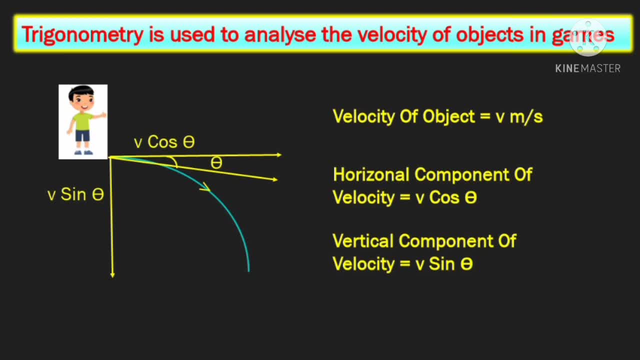 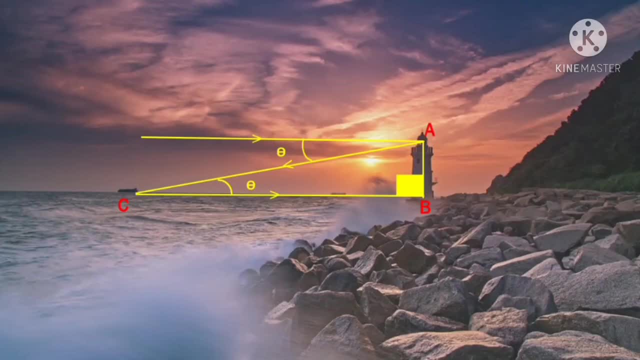 So trigonometry is indeed handy in video gaming. The next application of trigonometry is in navigation. So, friends, let's suppose a scenario where you have to measure how far a ship is from the lighthouse. Let's say the lighthouse is 60 meters in height and from the lighthouse you are observing. 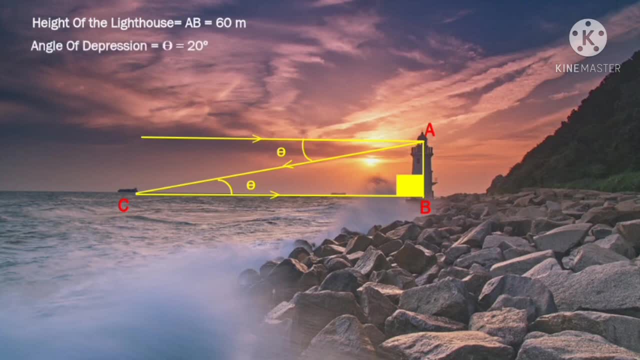 the ship and note down the angle of depression as, say, 20 degrees. Let BC be the distance of the ship from the lighthouse. So, friends, did you see that again you are getting a right angle triangle here. So again you can use trigonometry and say that tan theta is opposite upon adjacent with. 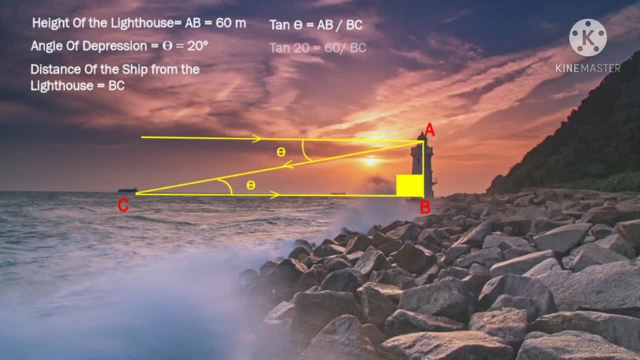 which is AB, upon BC. So just substituting the values, we will find that BC is nothing but 164.83 meters. So the distance of the ship from the lighthouse is 164.83 meters, and this is just one of the many ways in which trigonometry is useful in navigation. 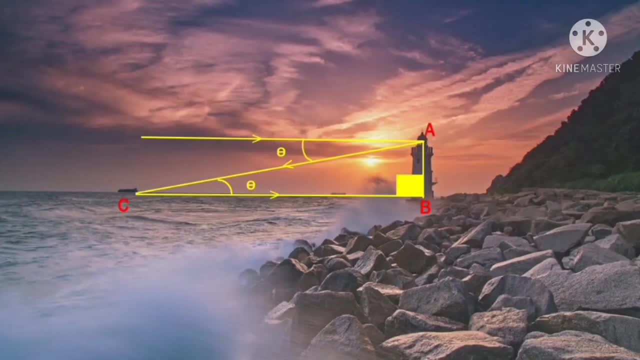 suppose a scenario where you have to measure how far a ship is from the lighthouse. let's say the lighthouse is 60 meters in height and from the lighthouse you are observing the ship and note down the angle of depression as, say, 20 degrees. let bc be the distance off the ship from the lighthouse. so, friends, did you see? 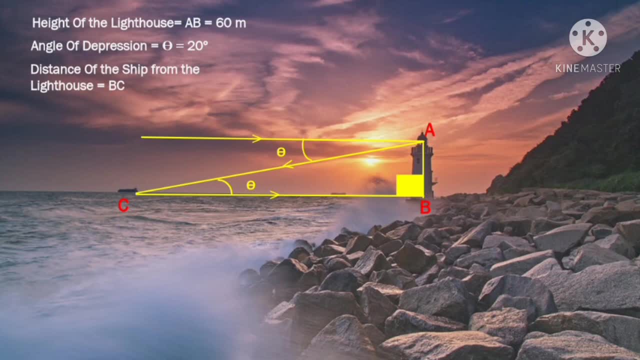 that again you're getting a right angle triangle here. so again you can use trigonometry and say that tan theta is opposite upon adjacent, which is a b upon b c. so just substituting the values we will find that BC is nothing but 164.83 meters. So the distance of the 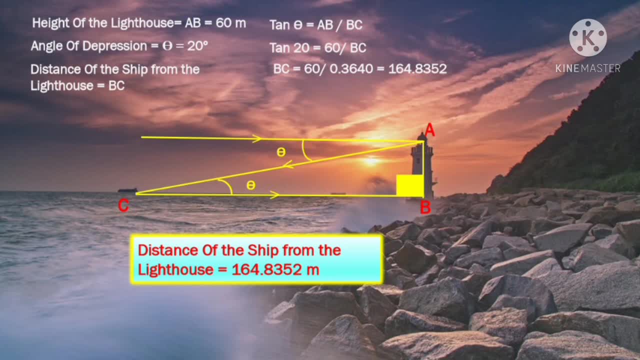 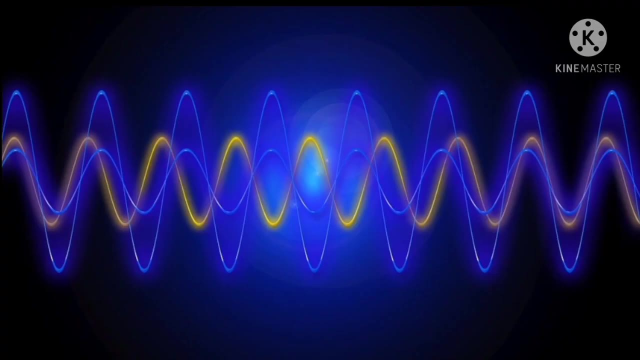 ship from the lighthouse is 164.83 meters, and this is just one of the many ways in which trigonometry is useful in navigation. The next application of trigonometry is in music. Now, that's surprising, but true friends, because music is nothing but sound waves, and sound wave can be represented. 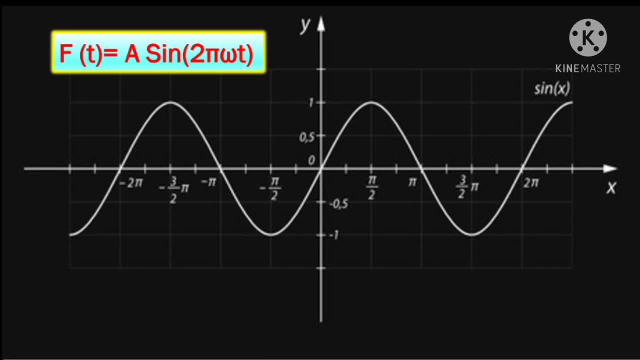 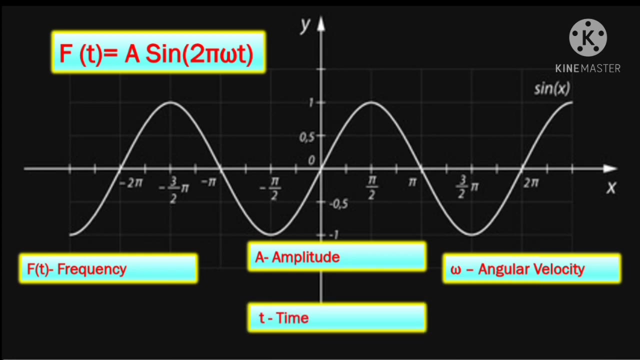 by this equation, f of t, equal to a sine 2 pi, omega t, where f of t is the frequency of the wave, a is its amplitude, omega is the angular velocity and t is the time. So by manipulating the values of angular velocity, t and a, you can make the wave taller, wider or narrower, and sound engineers use 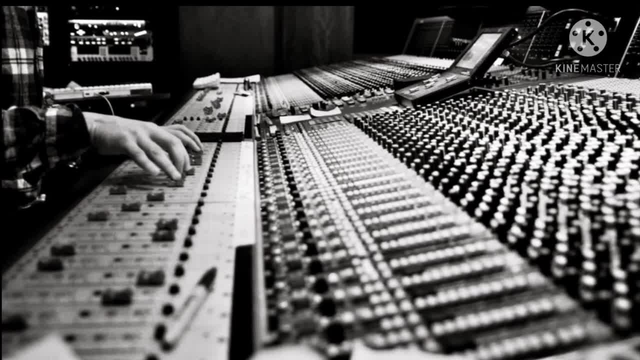 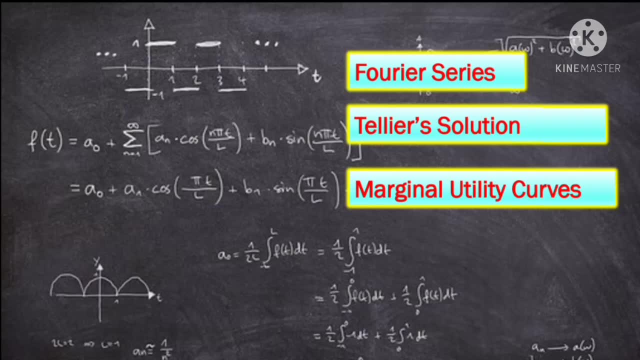 this property to create computer generated sounds, and a lot of trigonometry is used to create digital audio. So trigonometry is indeed very useful in music. Last but not the least, trigonometry is very useful in economics. So, friends, the main property of trigonometric 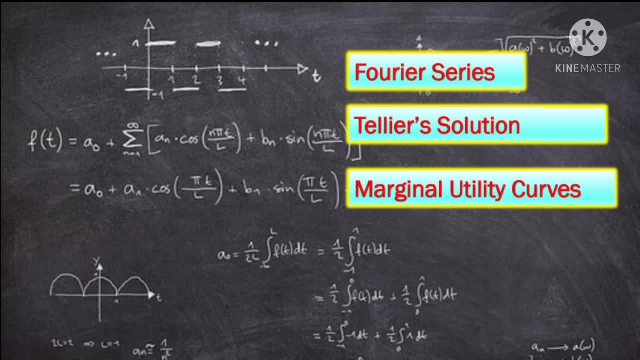 functions, as you might have observed, is that they are very cyclic in nature, So this property is used in finance and econometrics, while creating marginal utility curves. Also, the tellus solution and Fourier series are used in finance and econometrics And they both use trigonometry, So in this way, trigonometry is very useful in economics. 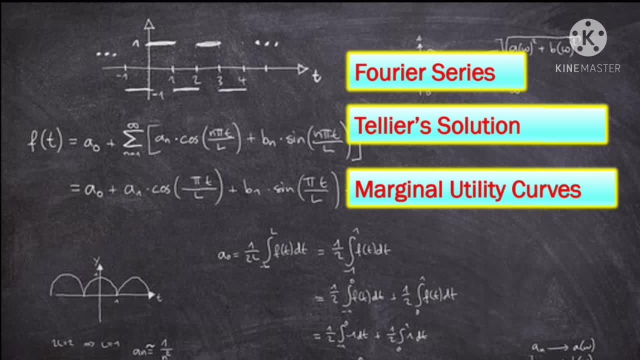 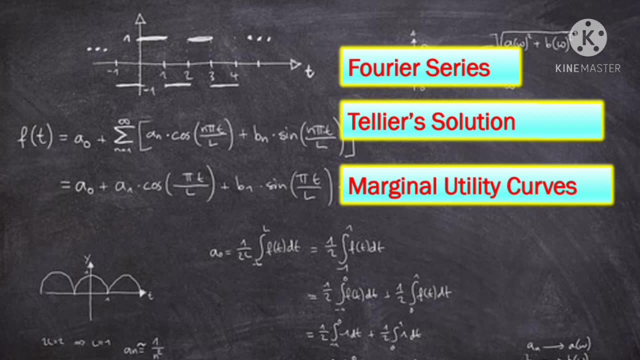 So, friends, I hope you found the video useful. If so, do consider subscribing to my channel. Do like and share the video, and do leave your comments in the comment section below. So till we meet again next time. take care, bye.